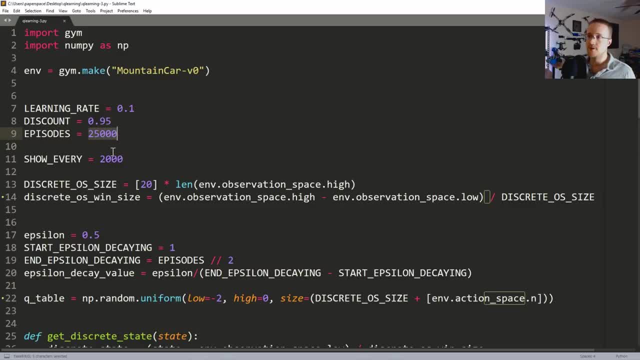 showing. let's say, even with 25,000 episodes showing every 2,000, that's still not a statistically significant sampling of how your model's doing. So we have to find a better way, and one thing that we can do- just a simple metric to track is just simply the reward. So a per episode reward tracking. 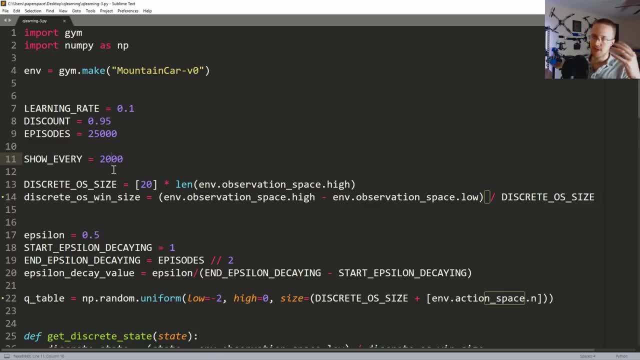 system is probably enough For most like basic operations. now for really complicated environments you might need to do a little more, but you're not going to use basic Q-learning for a complicated environment anyway. So with that, let me just show you guys one way you could track these, these metrics, over time. Now 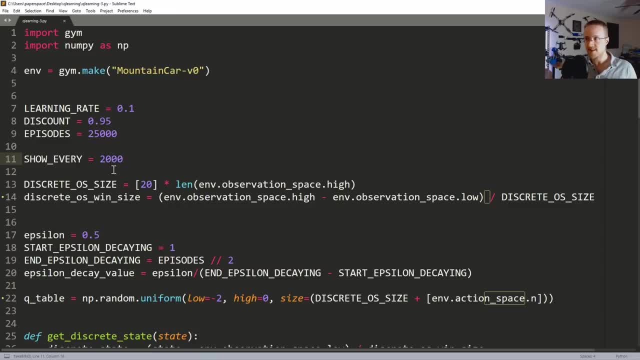 there's a million ways you could do. this is just a simple programming task, honestly, but it is something we definitely need to do. So I'm just going to show one example and then, after that example, I'm going to show you guys something kind of cool with the Q-table. I'm going to show you 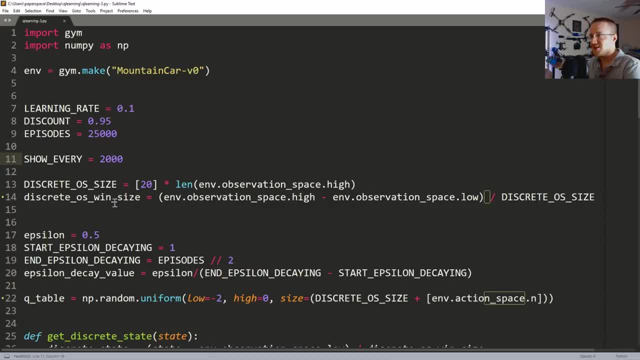 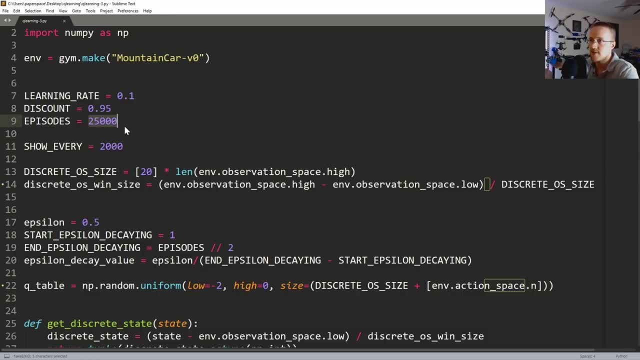 the Q-tables at the end as a just a slight bonus. So anyway, the first thing we're going to do here is just come underneath Q-table Also, let's change episodes, Let's do. let's just do 2,000 episodes, show every 500 episodes. That'll just help us to get through this year. So the first thing that 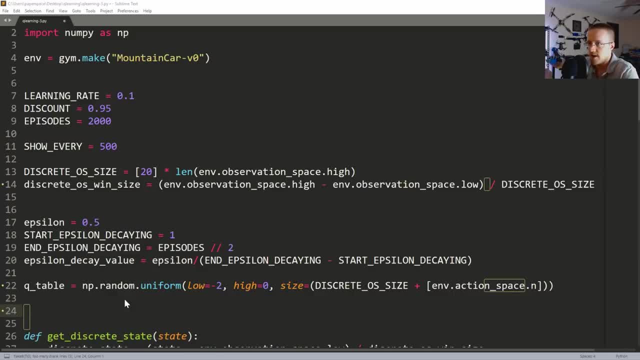 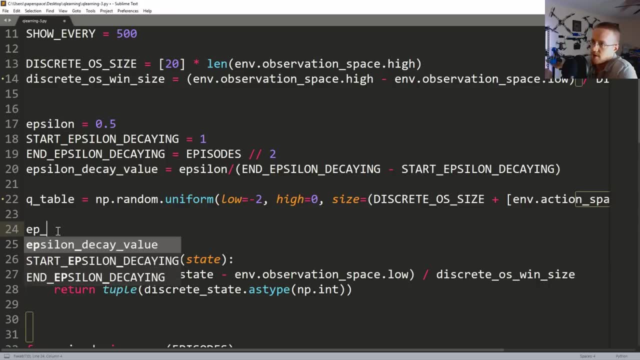 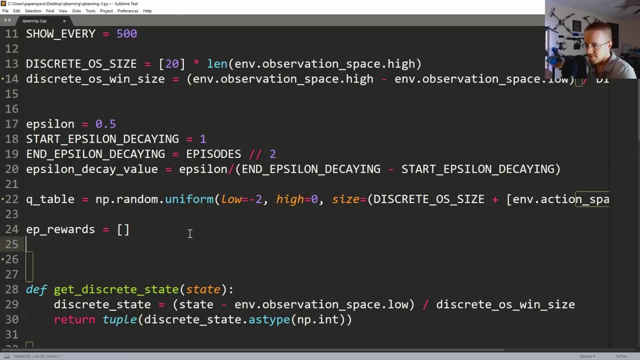 we're going to do is, just underneath Q-table, let's just create a couple of new values. I meant to just zoom in a little bit there. so, uh, first of all, we're going to have episode rewards. this will just be a list that contains, uh, each episode's reward, just as a list, uh, and then we're going to 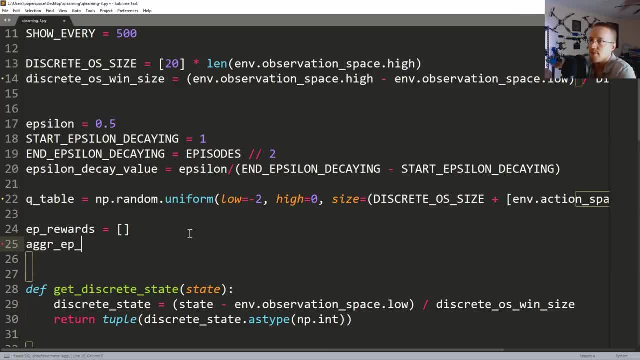 have an aggregate, aggregate ep rewards dictionary, and this dictionary is going to track, uh, the episode number, basically. uh, then we're going to have the average, and then we'll have the min, and then we'll have pep8 troubles and we'll have max. okay, so this is, this will just be- a dictionary that tracks. 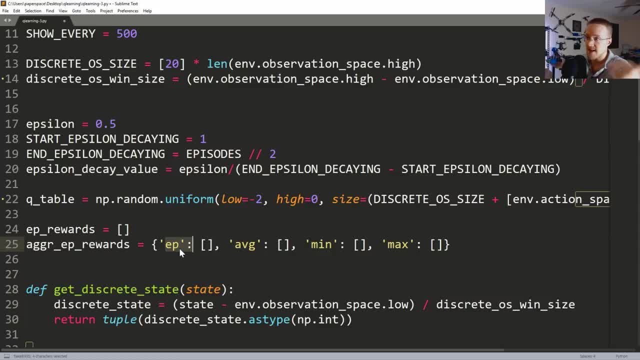 episode number. so this will just serve as like an x, yeah, the x-axis for a graph. basically, um, uh, the average. this will be the trailing average. so you almost think of it like, um, it's not a moving average, but it's the average for any given window. so every 500 episodes for 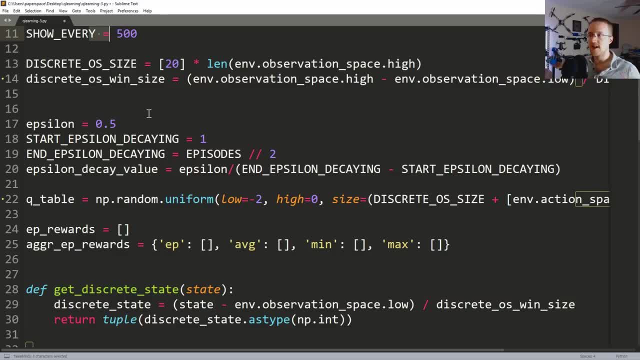 example. this will average over time, so as our model improves, average should go up, uh, minimum. this is just going to be tracking for every show, every what was the worst model we had? so um so, so basically it's just what's the worst. that's not a hard concept. 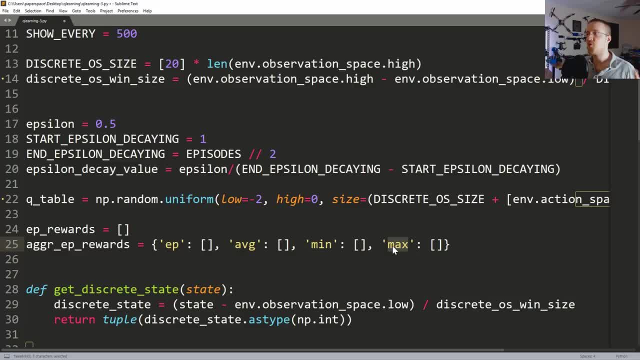 okay, max, what was the best one? so why do we want these? well, the average might actually be going up, uh, but the minimum or the worst performing model is still in the dump, and so you might have cases where you actually prefer that the worst model is still somewhat decent than to have a highest average. 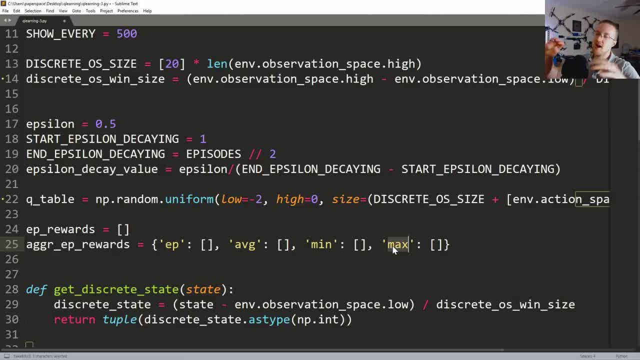 or something like that. so this is just barely getting into it. this is, you know, what you're going to actually be looking for. trying to optimize for is going to vary depending on what kind of tasks you're attempting to achieve, so i'm just going to keep it fairly simple here and just go with that. so the next thing we're going to 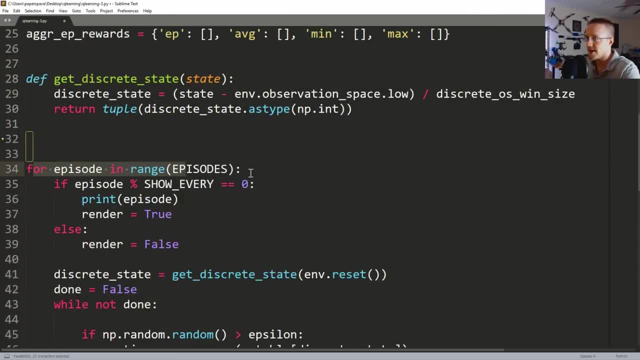 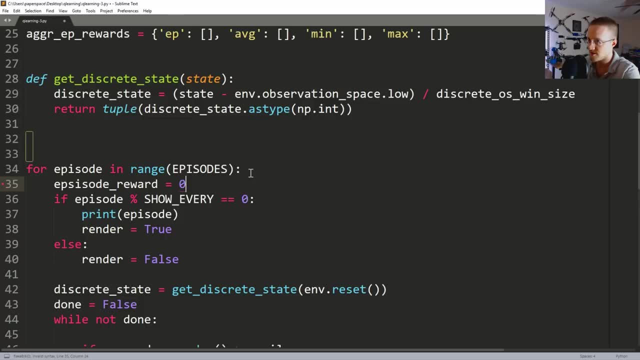 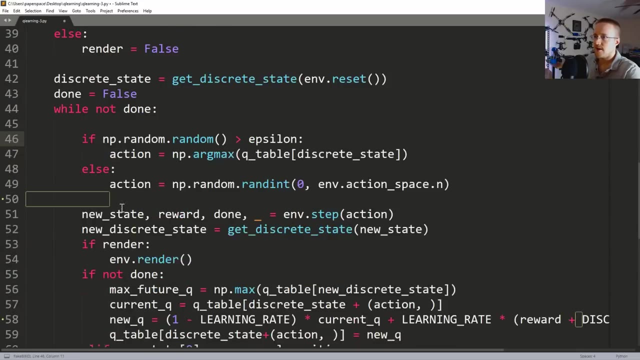 do is we're going to come down into the episode loop here and we're going to track episode underscore reward. we're going to say that equals zero. then we're going to come down to the iteration of steps uh, which is here, and then we get a reward here and what we want to do is add that reward. so 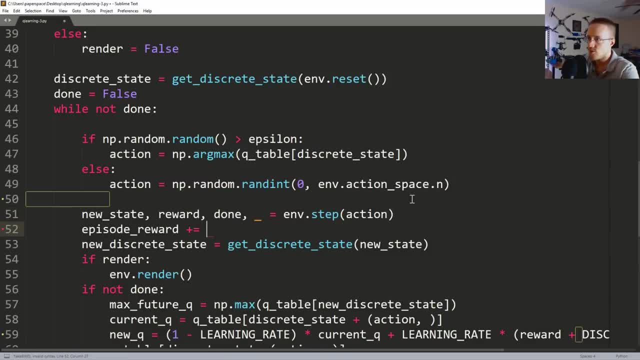 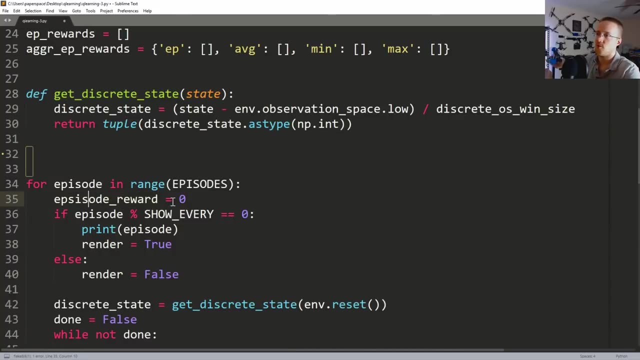 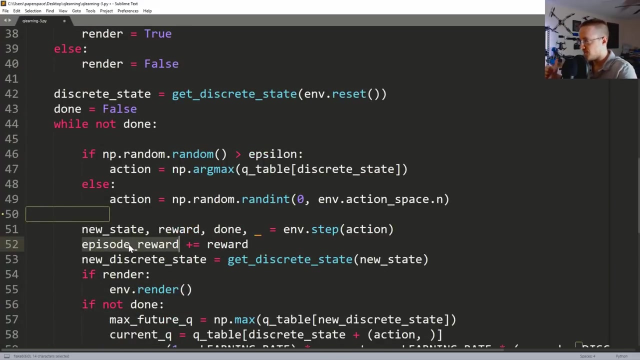 episode underscore: reward plus equals reward. uh, then, what we want to do? what's your deal? i guess because we're just not using it. yeah, undefined name episode: wait, whoa, epic. oh, we typoed episode reward. ep. episode episode reward. okay, coming down here. episode reward plus equals reward- phenomenal, okay, so that will add to episode. 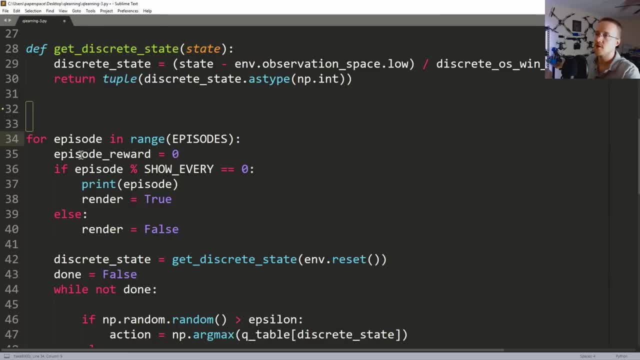 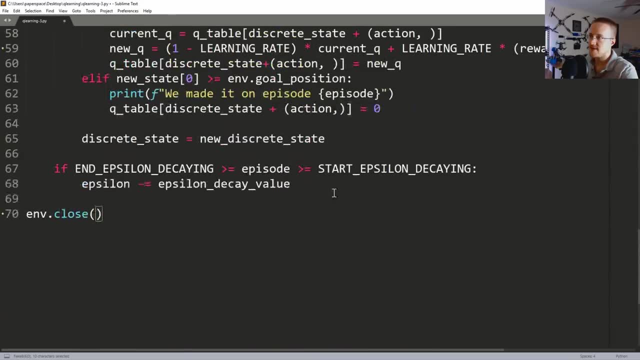 reward every time and then, basically, at the end of the episode, what we'd like to do is a pen episode reward to ep rewards. so we'll come to the very end of this loop, we'll come back here and the first thing that we're going to say is: ep underscore. 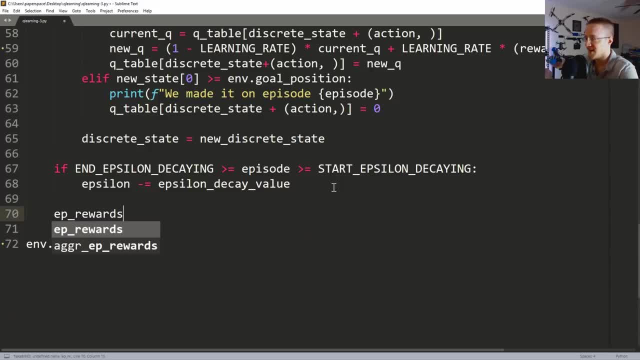 ep rewards. i don't know if my keyboard's dying or what. i'm pretty sure i didn't make that typo. uh, ep rewards dot append, although eps reward episode rewards is a little hard to explain with a keyboard issue. but anyway, ep rewards dot append. um, we want to. 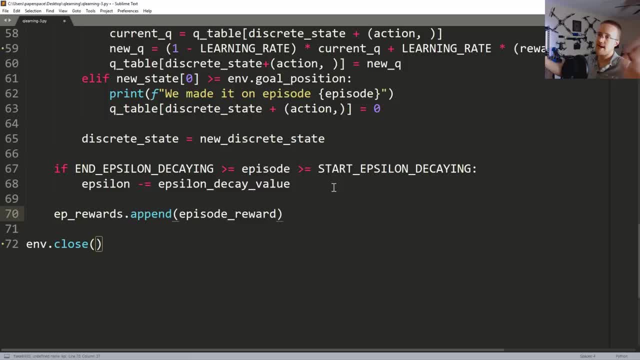 append that episode reward, so the total reward, at the very end. what do we want to do? so then, the next thing we're going to say is: if not episode uh, episode modulo, show every um, and that for just for the. that's the same as saying if episode modulo. 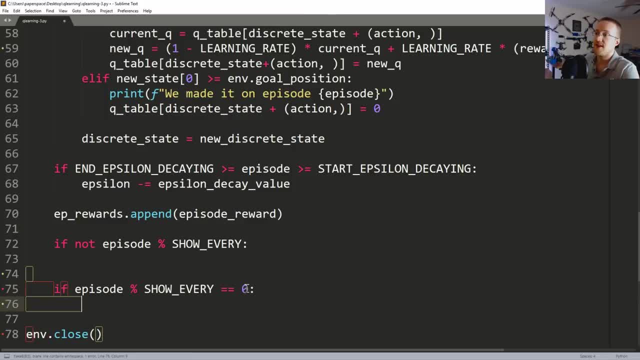 show every double equals zero. so if it doesn't equal zero, so you can kind of of shorten this just by saying: if not, episode modulo, show every. basically it just means every show, every, do this thing. so i can't tell you how many times in python i need to perform a task like. 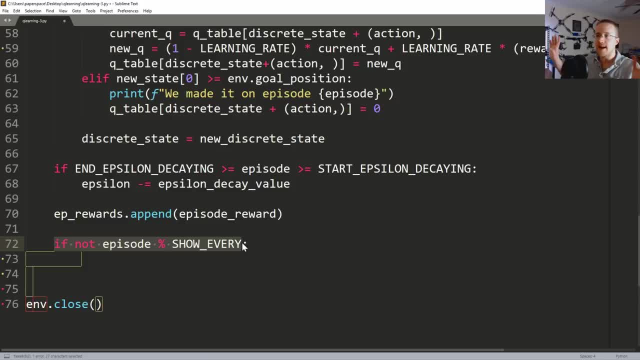 this and it's kind of unfortunate that this is the like industry standard. it would all, would be kind of nice to have some sort of way to be like, like, every like. wouldn't that be a nice statement in python, every just saying something like that. anyway, make it happen, guys, uh, if not? episode. 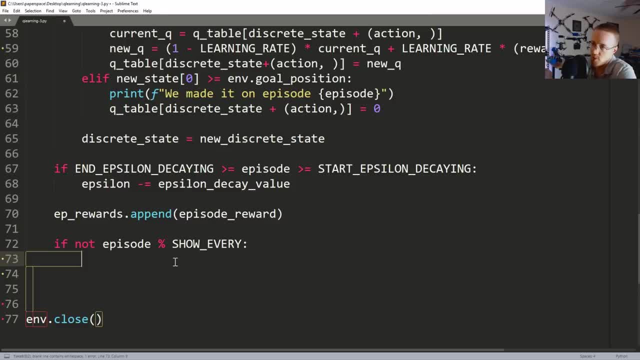 show every. so now, what we want to do is we actually want to build? uh, we're going to work on our dictionary, so, basically, first thing we're going to do is calculate the average reward, and that's going to be equal to the sum of our episode. 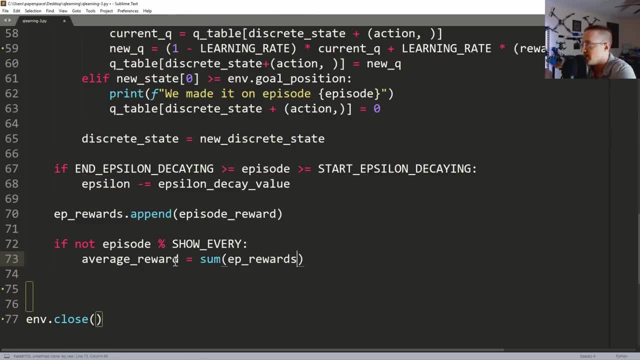 ep underscore reward. there we go. it'll be the sum of ep rewards minus the show every colon and then divided by. and i know some people are going to be like: why don't you just divide my show every? well? in this case, some like this: minus show every colon just means, like the last, let's say 500. but if the list is, 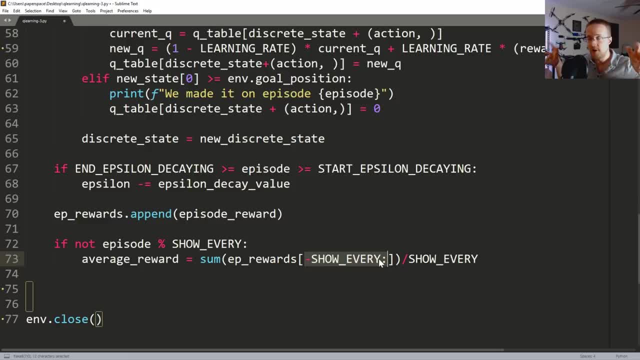 only 300 long and we do the last 500, it's still only going to be 300 long either way. we shouldn't run into that as a matter of fact. we should run into that as a matter of fact, we should run into a problem. but just in case, i'm going to instead say: the len of ep, rewards minus, show every cool. 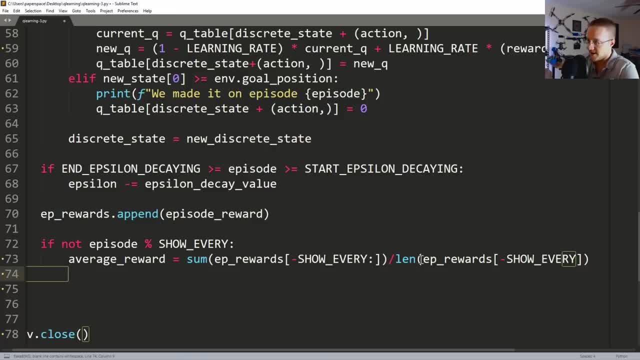 so that gives us our average reward, and now we're ready to actually populate that uh dictionary, so it was like aggregate ep rewards, and then basically, we're going to have um four things that we're going to do. first of all, the episode that's just going to be equal. 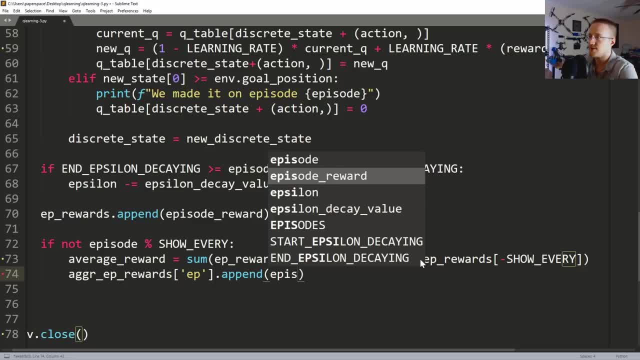 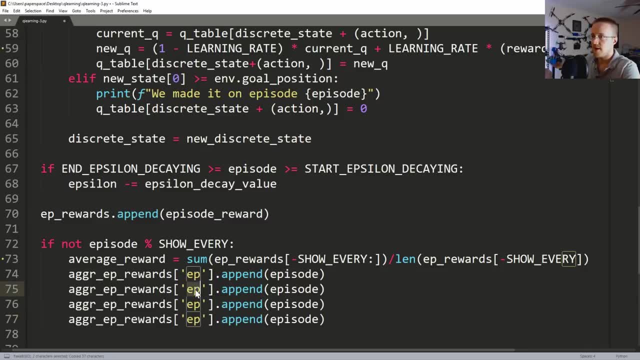 or not equal to. we're going to say: append episode, episode. and then i'm going to take this, i'm going to copy: pasta, pasta, pasta, average min and max. and so here we're going to append the average. then here i'm going to copy and paste. 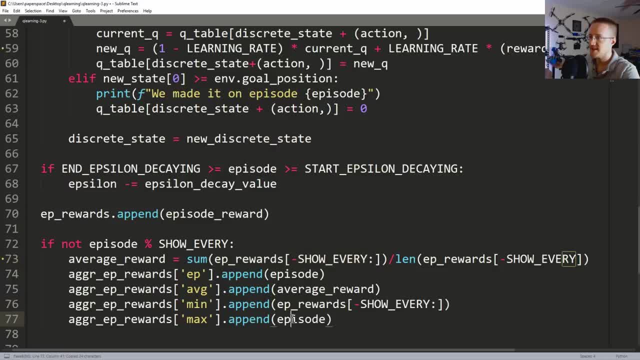 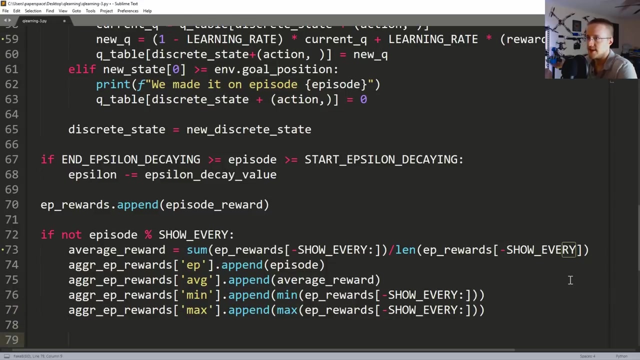 this upper words: minus show every colon thing, paste, paste. and this one will be: what was that? min, so the minimum of that value. and then here we're going to say: max, cool, beautiful. so now we've built, uh, this dictionary. the next thing that would be useful, possibly, is to: 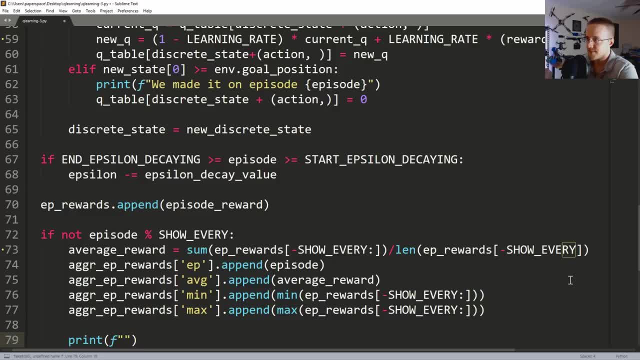 print an f string, um, so we can just just for this specific episode. we could print like all of these things so we could say uh, episode colon, uh, and then average colon, uh, min colon and then max colon, and then we'll just copy and paste into here, not cut copy, please. 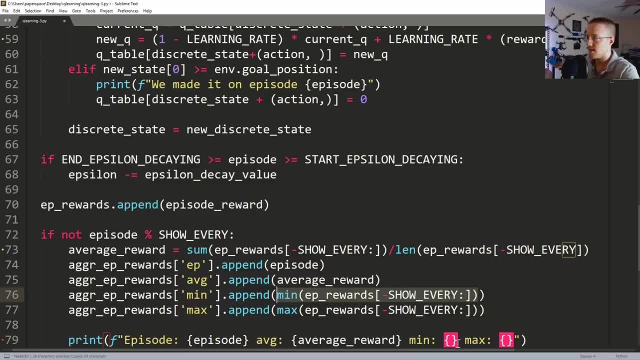 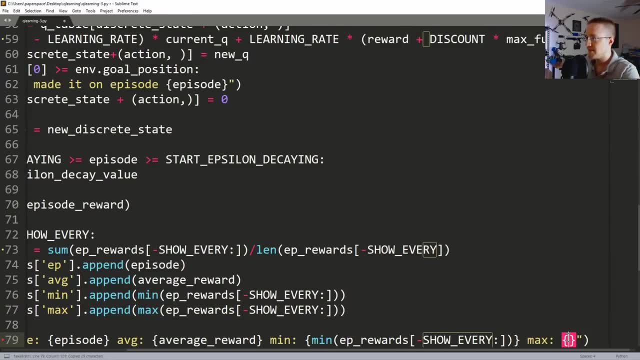 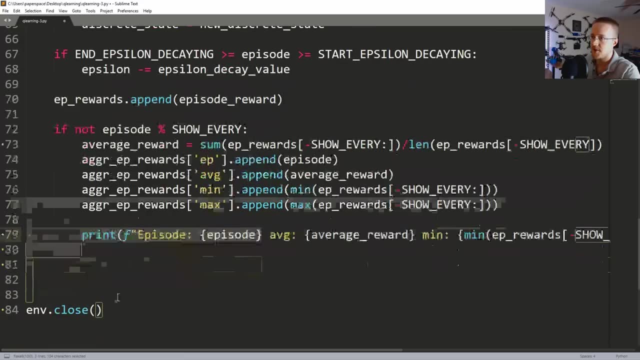 thank you. thank you, min max. so copy this, paste and then do the same thing for max here. copy paste, okay. so that'll give us some, some metrics, like as it's training for us, so we can kind of see how things are going, besides just seeing the simple replay, because, like i said, that's just probably. 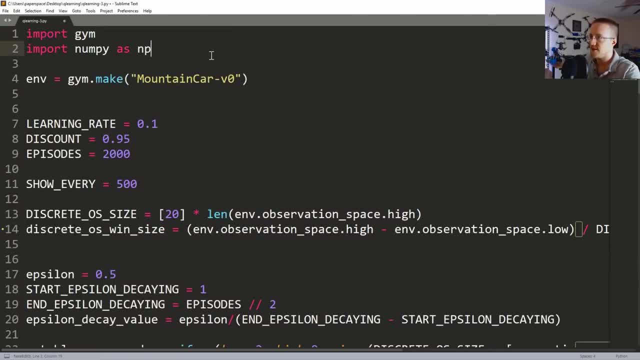 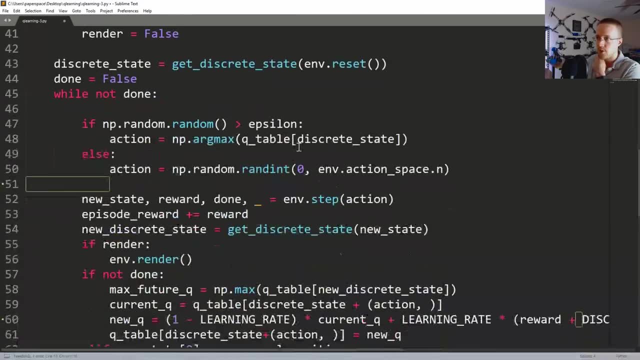 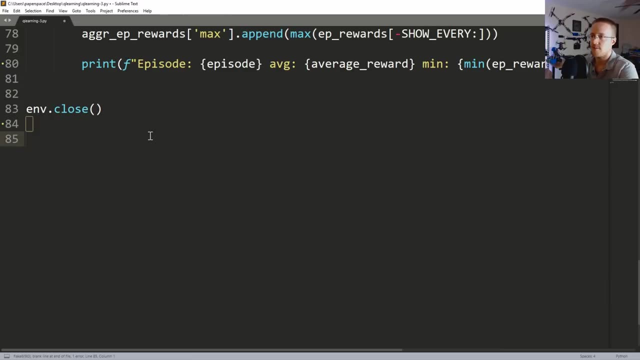 not going to be enough. uh, now, at the very end, we're going to graph it. so, at the very tippity top, we're going to import matplotlibpiplot as pl tizzle and then we're going to come down to the bottom again and um, again, we can close the environment, we. that shouldn't be a problem. so 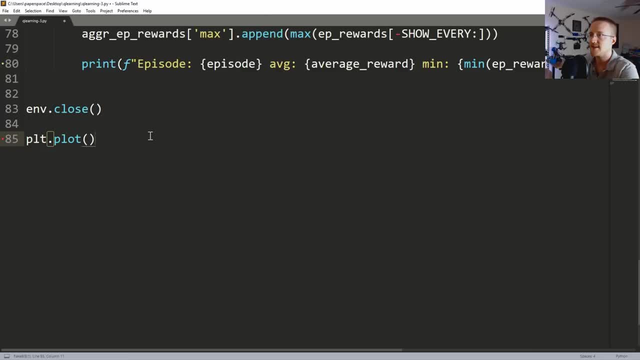 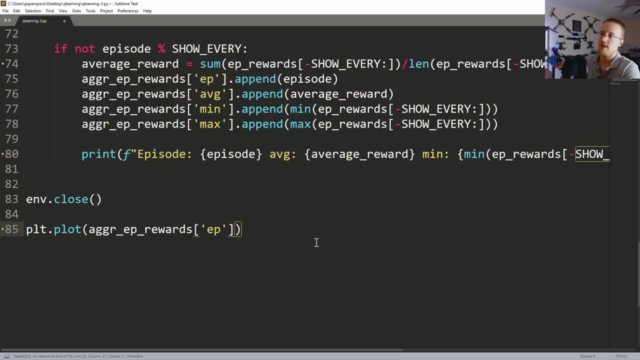 we'll do it here: plt, dot, uh, plt, dot, plot, and then we want to plot basically all three of these combinations. so basically it'll be the x will always be uh, the episode uh, and then we'll do avg, and then we're going to say: label equals avg, and then i'm going to copy this paste, paste, and then we'll do min. 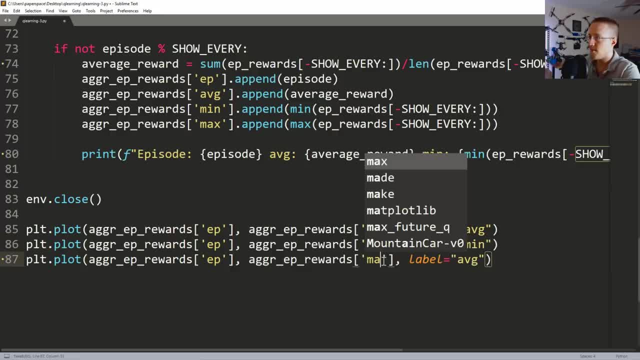 min. we'll do max, max and uh. then we'll do a plt dot legend and we'll say the location here is four and then finally plt dot show, and for the location, that just you can kind of pick where you want the legend to go. and i'm going to put it in four, which just means the lower right. so 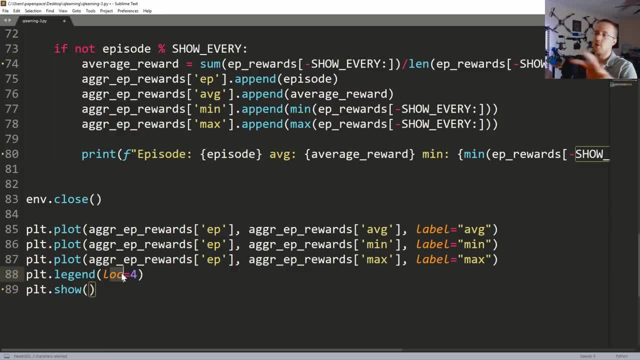 in theory, everything should be going up over time. so hopefully the lower right is going to be the lower right, and then we'll do max, max, and then we'll do a plt dot legend in the way- if it's in the way, we didn't do very well anyways. so so, anyway, we'll save that, uh, and 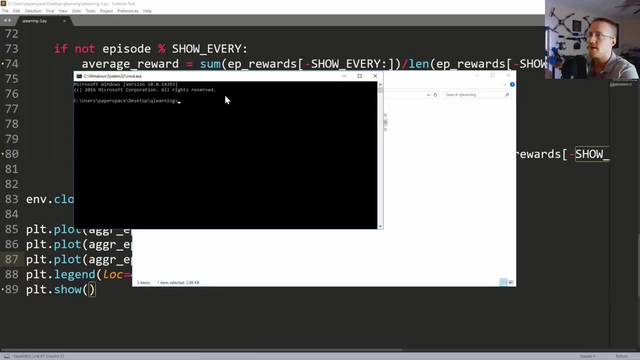 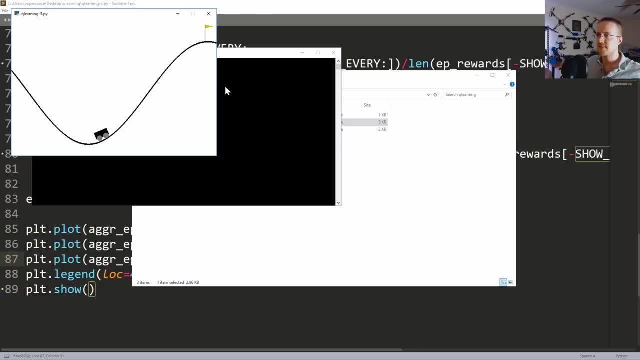 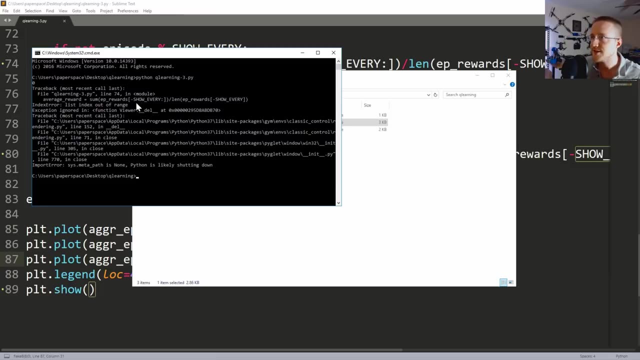 what i want to do is open up a command line, python q learning three. we'll get that at least started. um, i'm going to move this like here so we can hopefully see the metrics up. shoot is what i was going to say. list index at a. 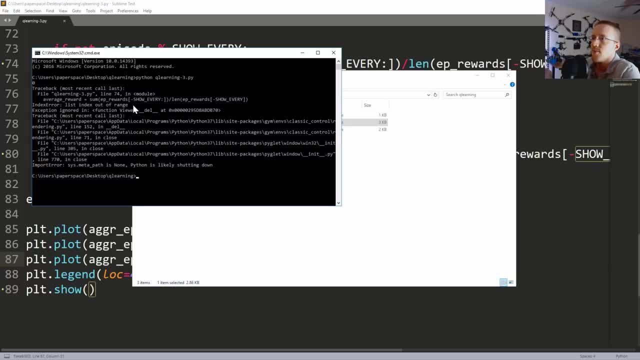 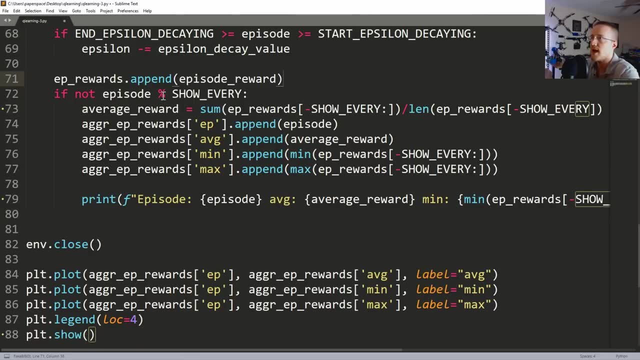 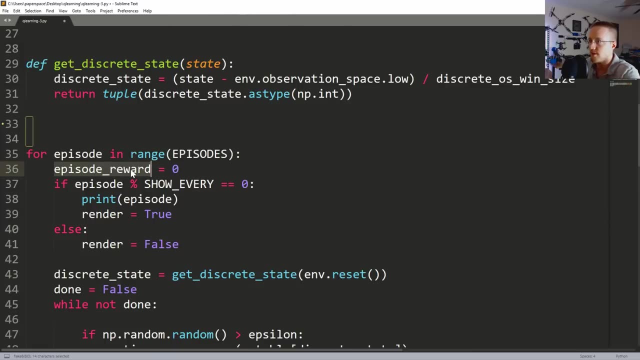 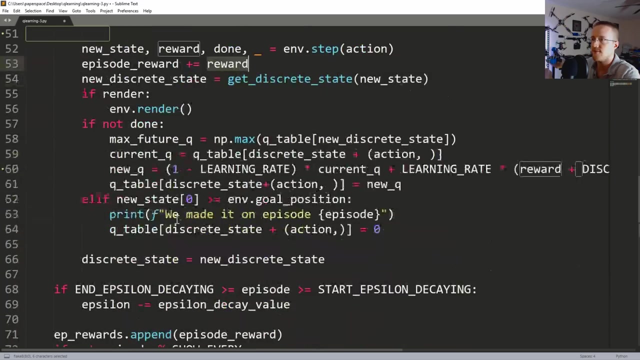 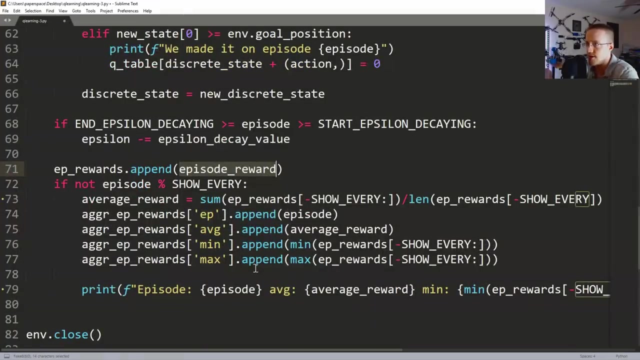 range f rewards, f rewards do we not append? uh f rewards, dot append episode reward. we are appending. uh, we've must have done something stupid. episode reward equals zero episode reward plus equals reward at the very end. f rewards dot append episode rewards. uh, then hold on um. i'm just not seeing what the issue is here. 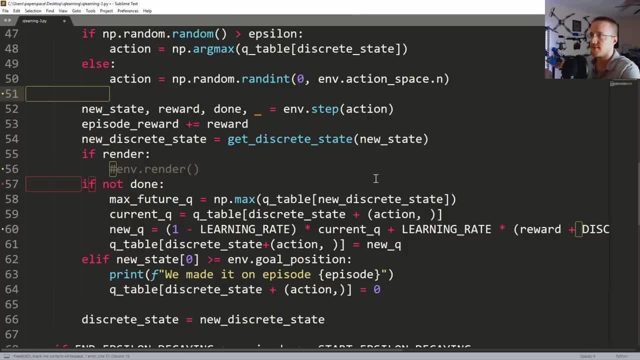 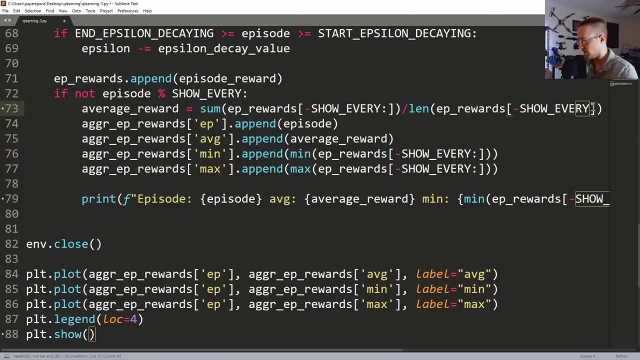 list index. oh, minus show every. okay, i see it. i see it. so, yeah, coming back down here. so the issue was: minus show every colon. uh, simple error. let's just make sure we didn't make that anywhere else. okay, so i think we're good, so let's try. 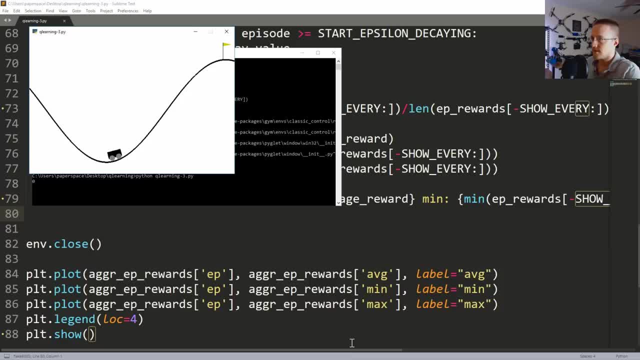 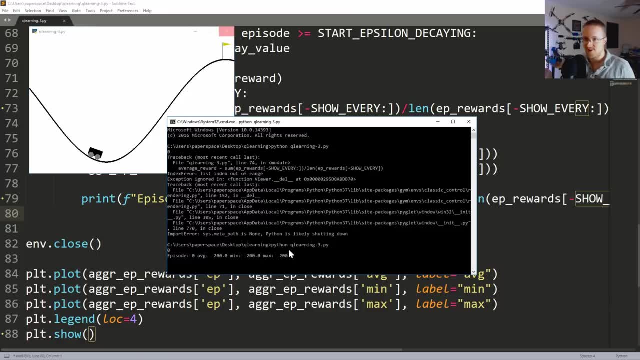 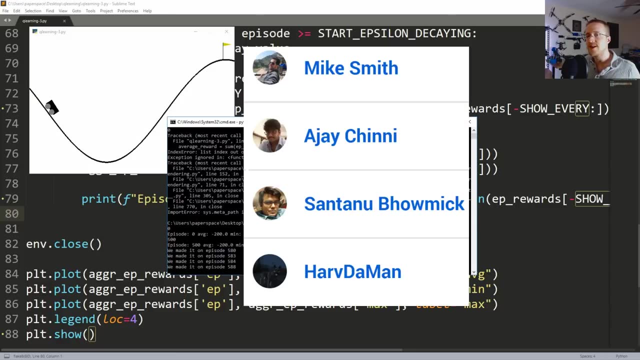 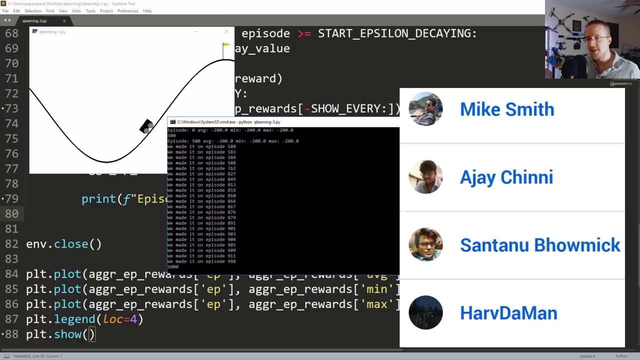 one more time. cool, okay. so everything's negative. two hundred here, uh, not two too shocking. so, uh, while we wait for this to do what two thousand episodes? i'm going to give a shout out to my most recent brand new channel members: mike smith, aj sheeny, santa, new bow mix and a hard work in the spring. no love on the best stuff. あ pra. 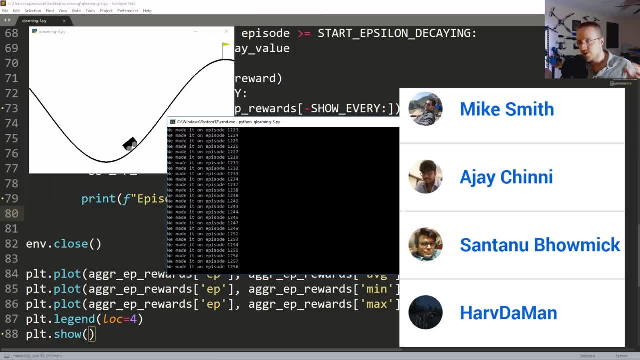 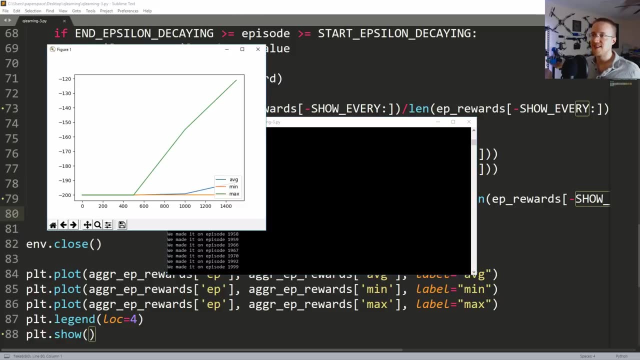 and harv demand. thank you guys for your support. welcome to the club, you guys are awesome. so it looks like: uh, we are almost done at 1500. wow, that stinks. he like almost made it to that flag. uh, okay, hopefully at this point we'll get a beautiful graph. wow, look at that. look at that. 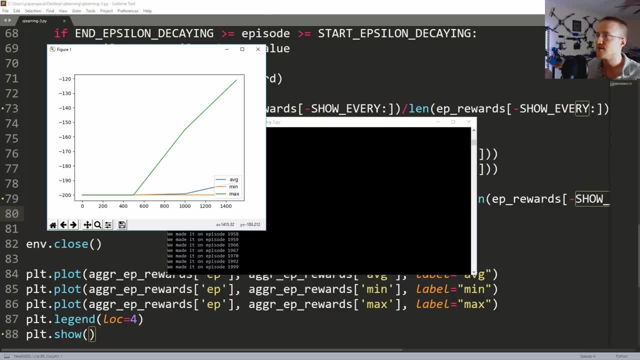 what is that average or max? i can't even tell. i think that's average or that's max. rather, of course it's max. it's the one that's on top. i was just testing you guys, to be honest. um, okay, so we can see here that things are improving. now. we only did 2000 steps, so it's no surprise that, um you. 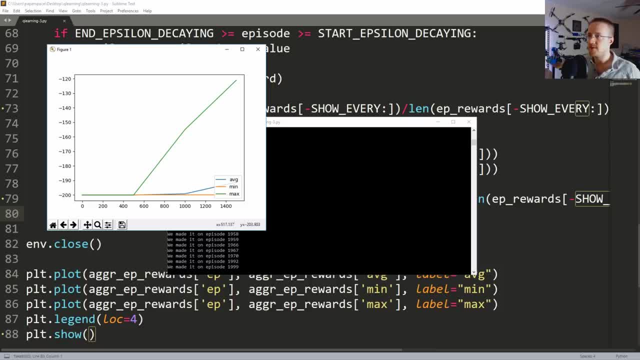 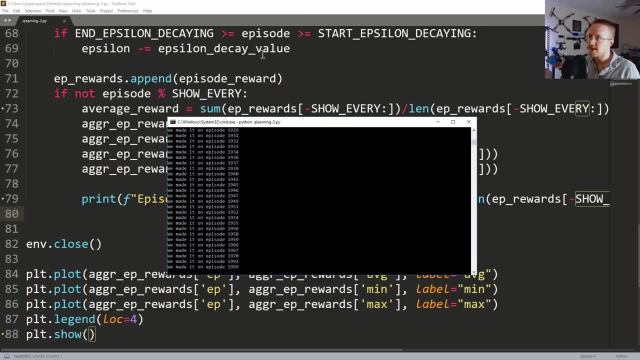 know the max episode was doing pretty good, uh, but the minimum is still going to be negative 200, like it just never made it to the flag. now, uh, we could continue. i'm just not going to waste y'all's time and, like you know, graph a super, really long one and just wait for things to iterate through. 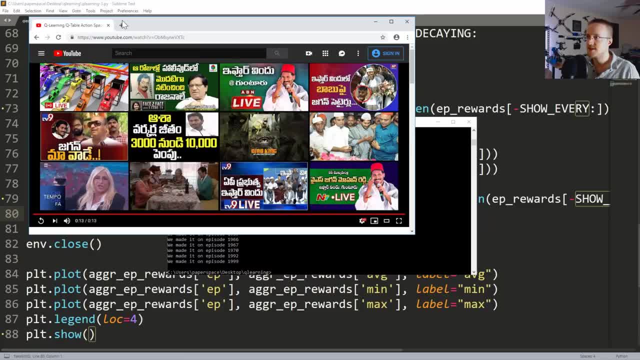 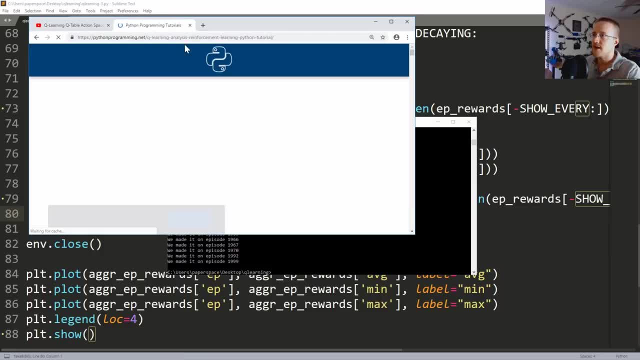 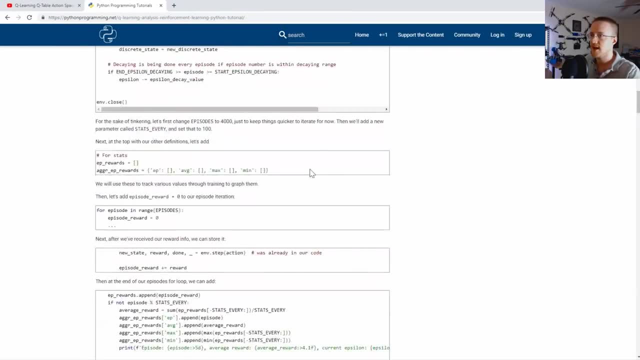 i've actually already done it, so, um, so, this is uh. well, this is a video i was going to show you guys, and i'll still show it to you. i'll just leave it in a different tab and instead we're going to pop over, uh, here, and i'm gonna, let's just full screen this thing and i'm going to scroll down so like. 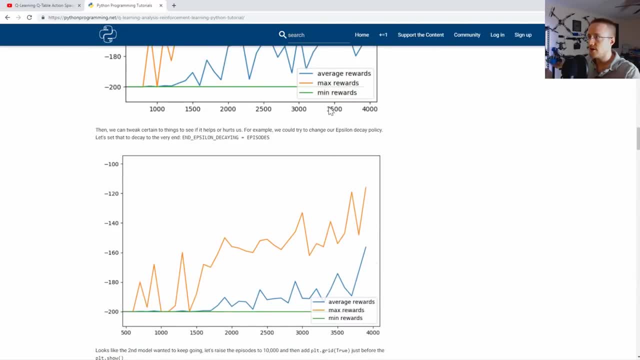 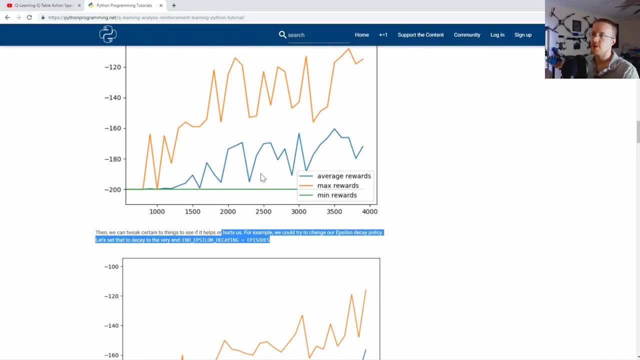 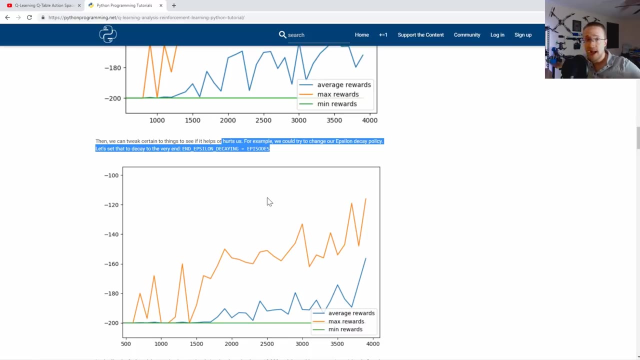 this is kind of basically what we were just looking at, and then i went a little longer. um, actually, i'm not even sure what did i change here. oh, this was just with an epsilon change. so one of the things that you would use these graphs for is like changing, like how does changing the epsilon uh, decay value? 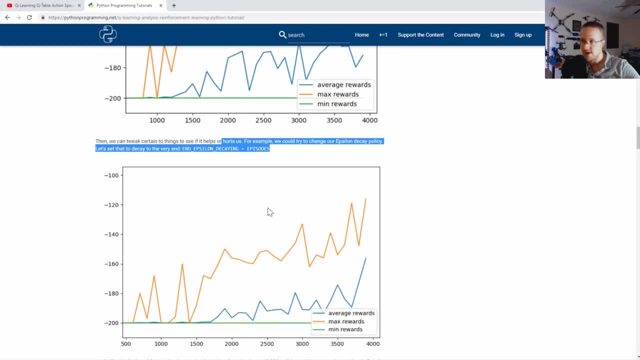 change. how does the start and stop, uh, episode number change things, all that kind of stuff. and also you can train a model for a little bit without an epsilon. then add the epsilon. how does that change things? like you could do all kinds of stuff like this is totally up to you what you want. 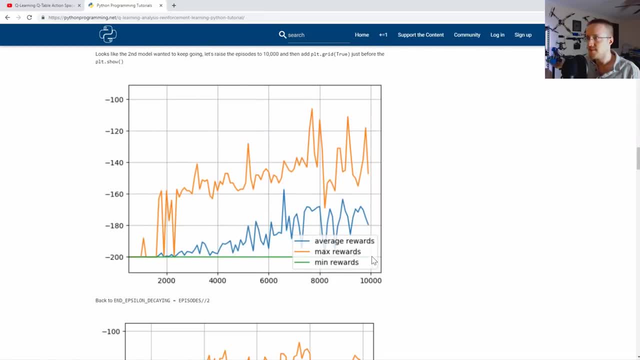 to do so. then even after 10 000 episodes, you can see the minimum for you. like i said, it got in the way because it didn't do very well, uh, but there is a little tick up right here where the minimum was at minus 200, but hey. 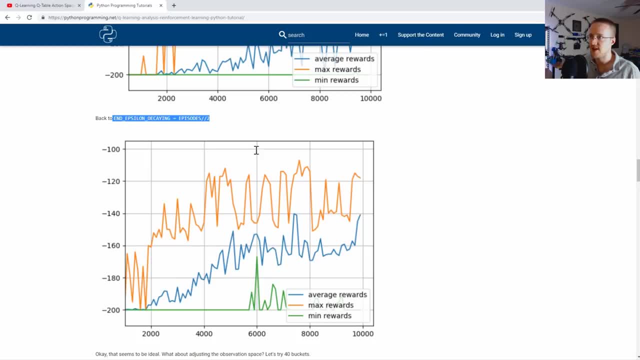 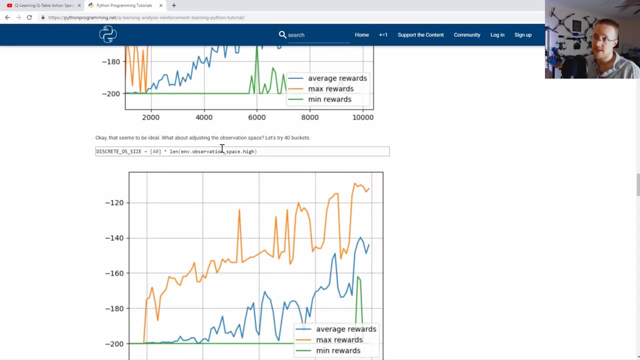 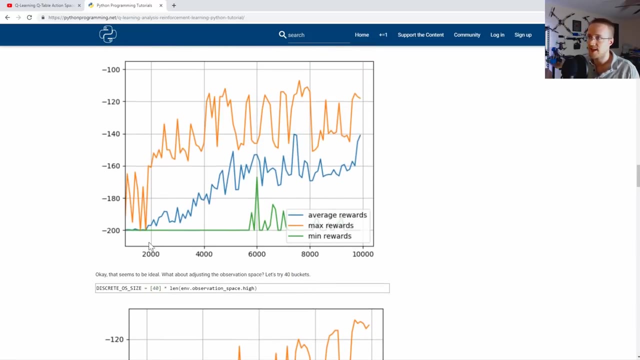 uh, and then again. uh, this was back to changing the epsilon decaying value. you can see how that changed some things. uh, then here i changed the discrete observation size from 20 to 40 and we can see here that at least the improvement is like super linear, like here you can see it. 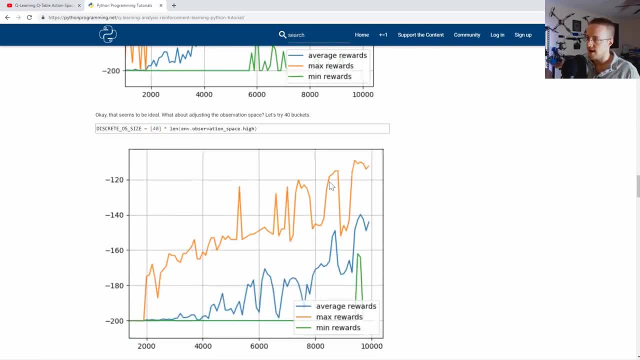 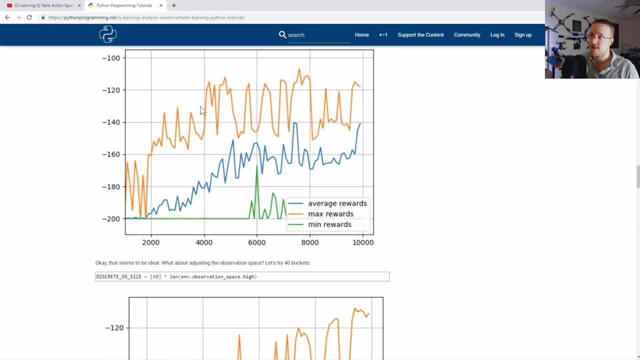 it goes up, but then it kind of flat lines, plateaus, uh, whereas here it definitely is improving, like to a point in continuing past- or at least we. it looks like it's gonna, uh, continue past any other point we've ever had, and for the same number of episodes. so then i'm like okay. 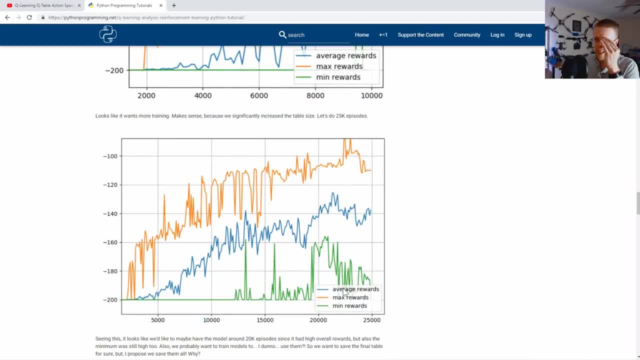 let's train it for really long. so we did 25 000 episodes and we can see, maybe at least for this setting, the sweet spot's around 20 000, because we can see the the worst agents were still, uh, at least making it to the flag, because if they don't make it to the flag, it's going to be a. 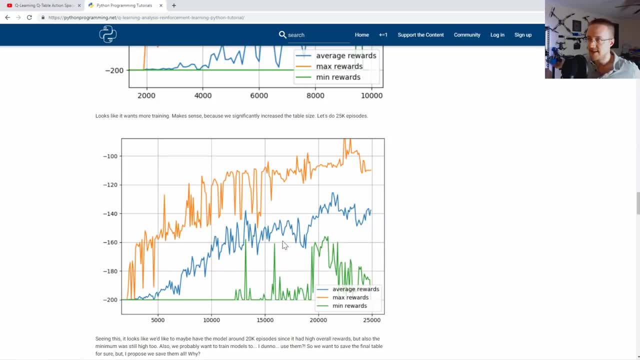 minus 200. so as long as they eventually make it to the flag, it's going to be a minus 200. so that's pretty good. so for you know, after about, you know, just before 20 000 to, i don't know, maybe 22 000 or something, um, for 2 000 episodes we found, or more than 2 000 episodes, i mean. 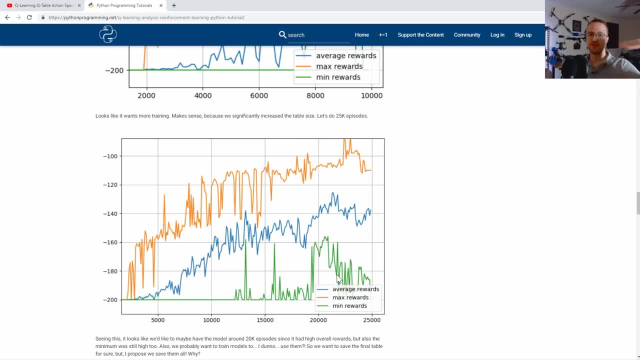 probably 3 000. um, it never failed. it was successful every single time and then, for whatever reason, it starts to come back down again. so, um, anyway, so you can kind of see how things changed, and then from here you can start tweaking like the epsilon value, or you could. 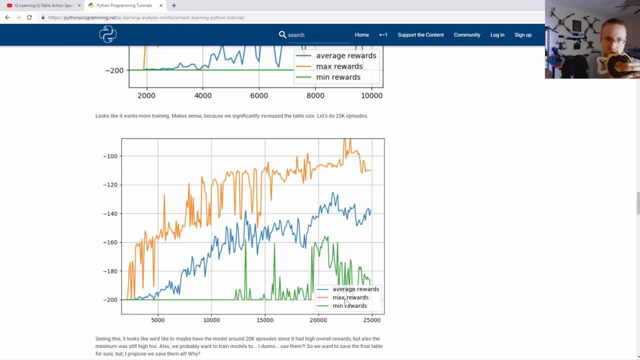 reintroduce epsilon, because chances are by this time the epsilon's not there anymore. so maybe we want to reintroduce epsilon because maybe the, the agent, is finding itself in a position it's never been in before, so that value has like never been tweaked, right, so stuff like that. 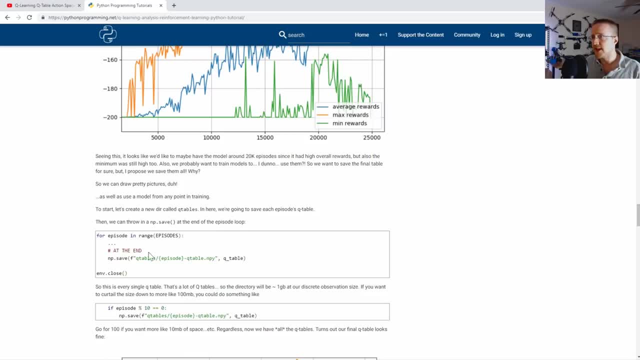 um, okay, and then here um is where we start talking about saving for q tables. so basically it's just a numpy save and then you can just save the q table as whatever you want. so for example, i'll just: well, yeah, you could save per episode, but that would be a lot of q tables. so instead, what i'm doing here, 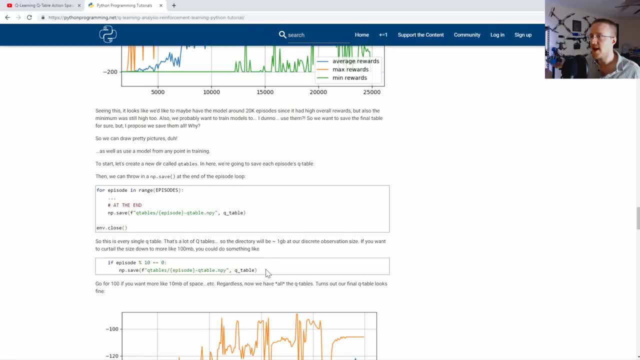 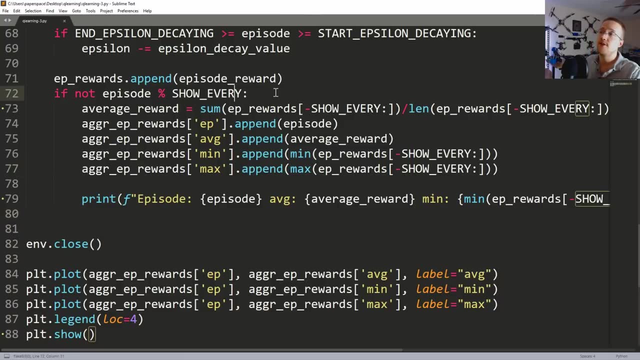 is that modulo thing. so you can, you could decide. you know, hey, i want to save, so, for example, i'll just take this, i cut this. uh, come over here. you know, basically you could save a q table, every show, every, so you could paste this in. you could say, okay, if you had it, we don't have the q tables. 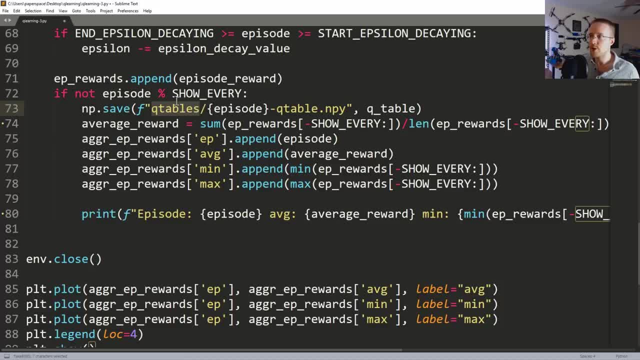 directory, but i made one in the text-based version. make a q tables directory. you save the episode number and then you can save it, and then you can save it, and then you can save it, and then you can save the q table there and you could just do this. so you could do this every episode. you could do. 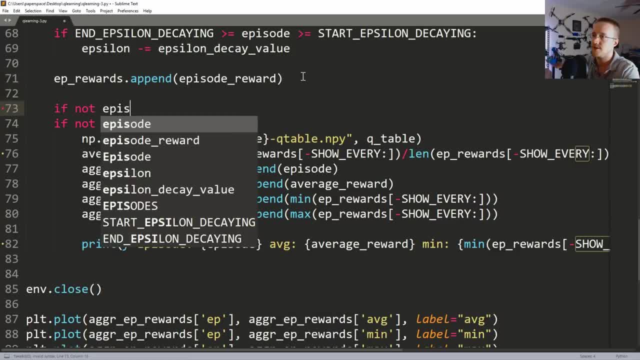 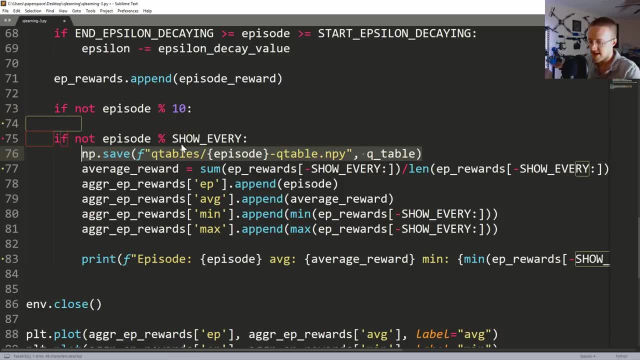 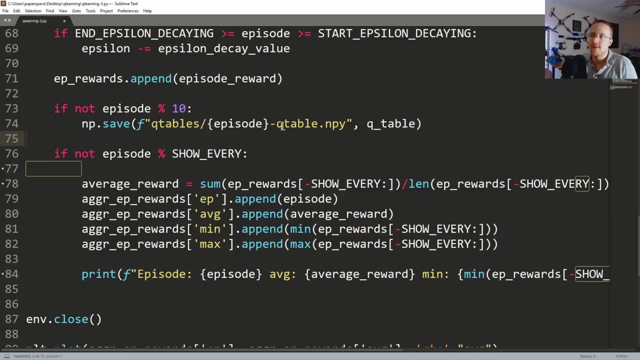 this every show, every, or you could say, if not episode colon, or i'm sorry, modulo 10, okay, and then you could instead save that. so in this case, it would save the q table every 10 episodes. uh, so it's really up to you how you want to do that, and you don't actually need to do that, but you would. 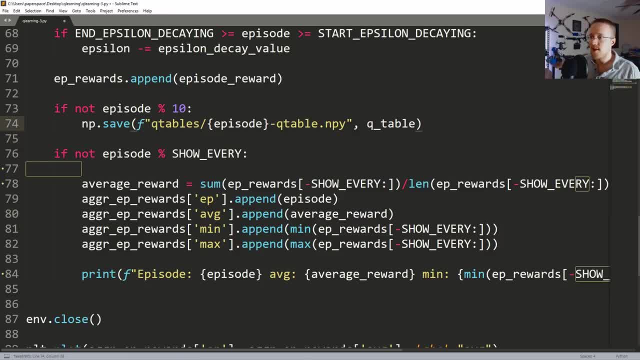 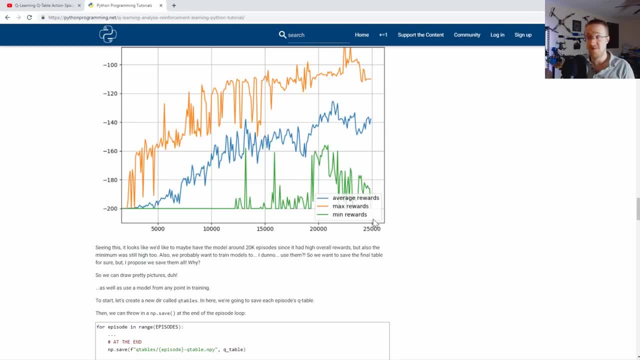 do that if, like, if you graph so like. for example, after i trained this model, it was clear by 25 000. well, it kind of went back to having some failures. so what i would have wanted to do immediately after having some of these failures be like: no, i want the model at 20 000, like that's. 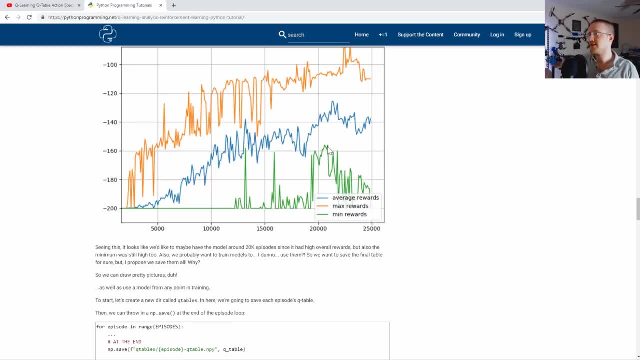 the one i want, or i want the one at like 20, i don't know, 21 000. it looks like i want that one. if i hadn't like, if i only saved the q table at the very end, too bad. now i gotta retrain, i guess. 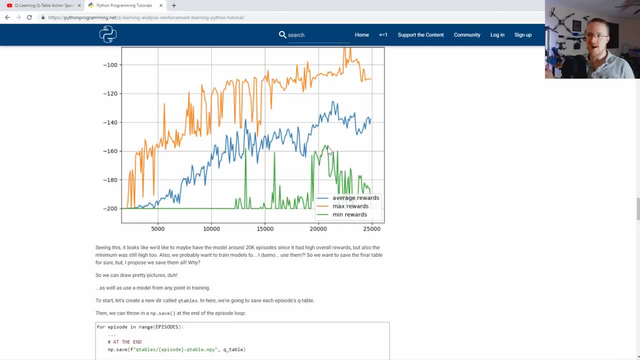 all the way to 20, and who knows if it's gonna look like that again, right, because there's a high degree of randomness here. so so that's one reason you might actually want to save the q table fairly frequently. you probably don't want every episode, but maybe every 10 or every hundred. but the other reason you can save 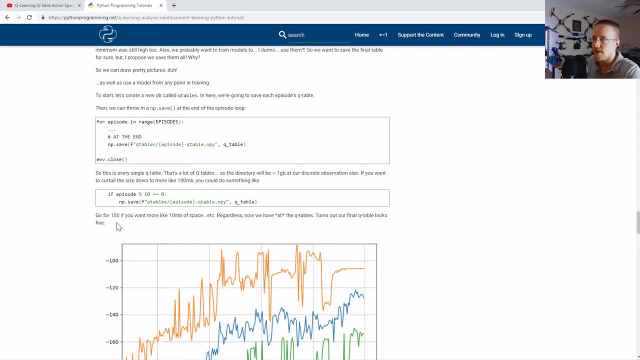 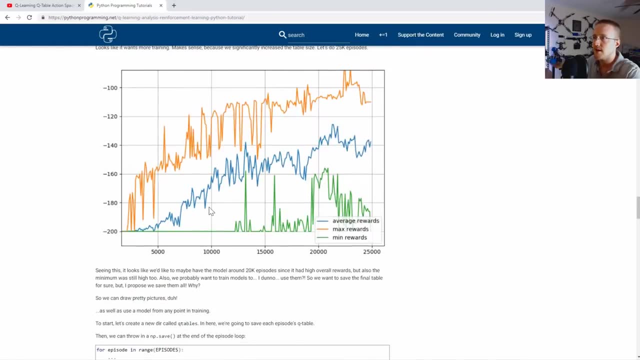 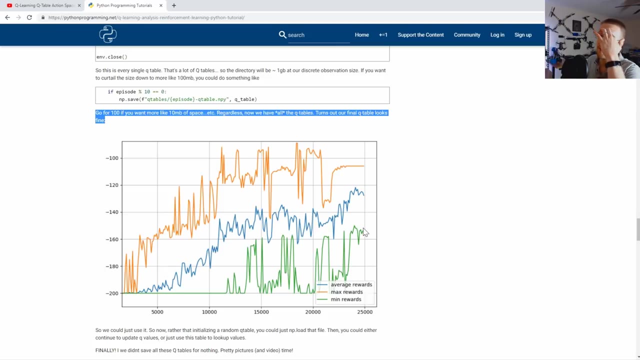 the q table um is. i'm curious what happened here. go for 100. i'm not sure what changed here, so we could just use like what's different about this one um than this one, unless it's just like doing it again. this one looks really good though. anyways, i'm not sure what changed for this picture. 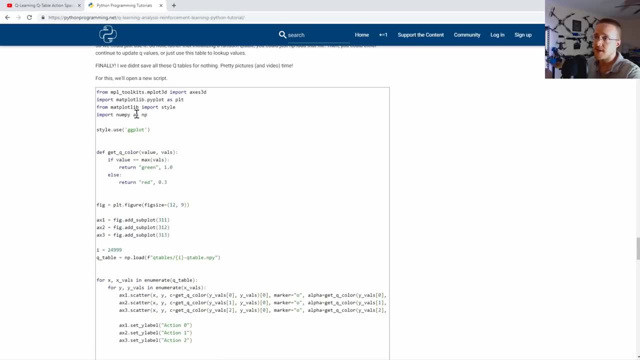 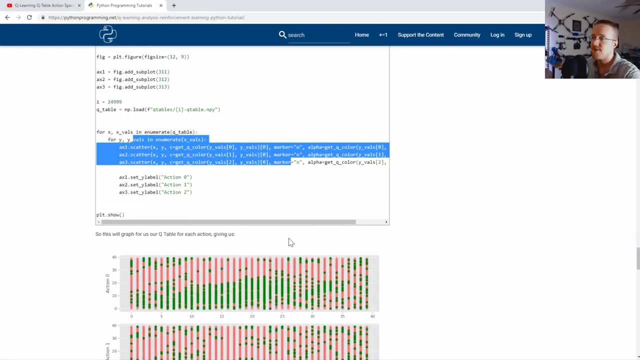 anyway. um, so once you have the q tables- this is what i did to generate graphs of the q tables. so in this case you can see i'm going to say i equals 24 999, so basically episode 25 000, because they start at zero. uh, then i just graph the q table, basically. so what we have here is the q table. 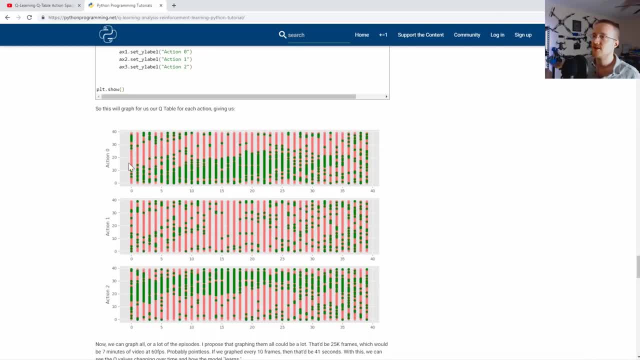 don't forget, i made the observation space a 40 by 40. so for action zero, this is your um, your all of your q values basically. well, not q values, but basically what i did is, if the q value is the max q value for each of the possible actions, i marked that, that combination, with a green dot, otherwise it's a. 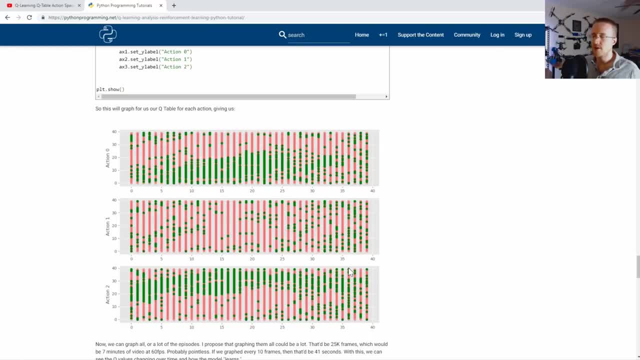 red dot. so you can see here, over time i also probably could have just kept it a green dot, but whatever anyway. um, my initial plan actually was to create a 3d chart and then, um, and have like cubes basically, and i started to do that and then it actually wasn't as cool as i thought it was going to be, and then 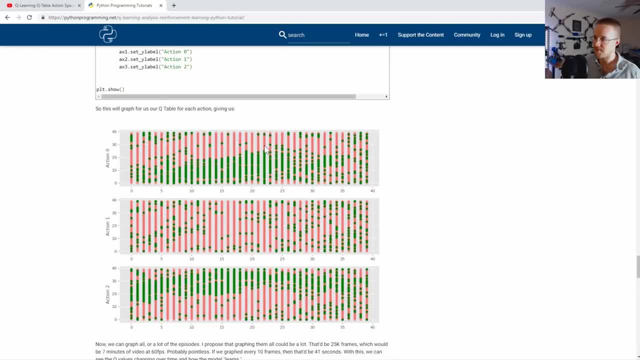 i was like: well, i could just graph like each of the actions and this is kind of what i came up with. so this is at the very end and you can actually see here action zero. that action zero was, i think, push left. action one, if i recall right, is just do nothing, and then action two is push right. so 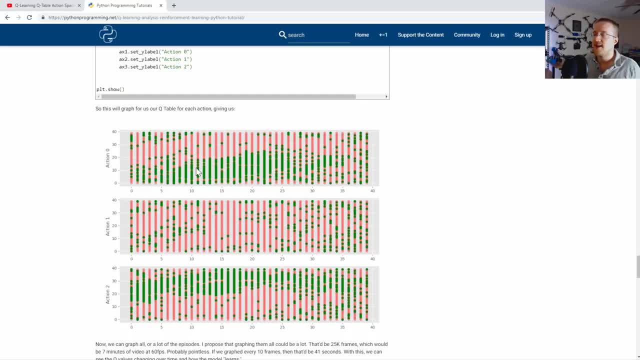 you can see, in these kind of this cluster here it's like this is pretty much always a push left and like some of these that aren't pushed left are actually probably just those, are still just left over from the random initialization and we just haven't hit that combination yet. 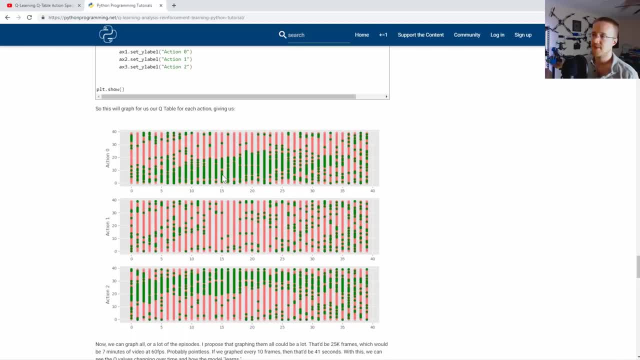 uh, it's probably what's going on there. um, and then here again, i can't imagine many circumstances where you wouldn't want to be pushing one way or the other. i mean, there's probably some like as you come up, like maybe you only want to go so high up the hills, or something like when you're swinging. 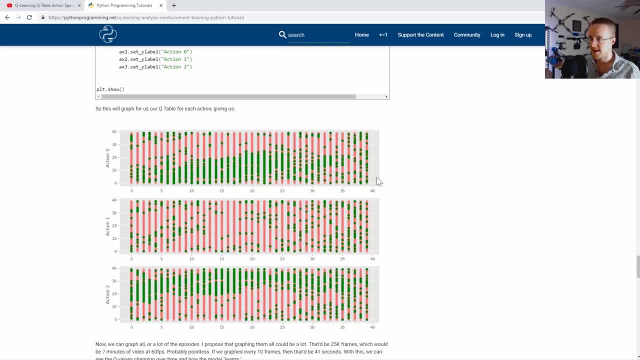 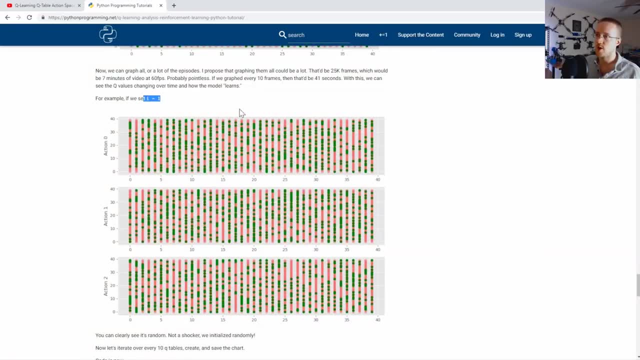 back the other way. so maybe that's it, i really don't know, uh, but anyway, so you can see how. anyway, it creates these little clusters, which is kind of cool. and then here this is: i equals one. so basically, after one episode, this is what it looks like. so obviously it's pretty random. 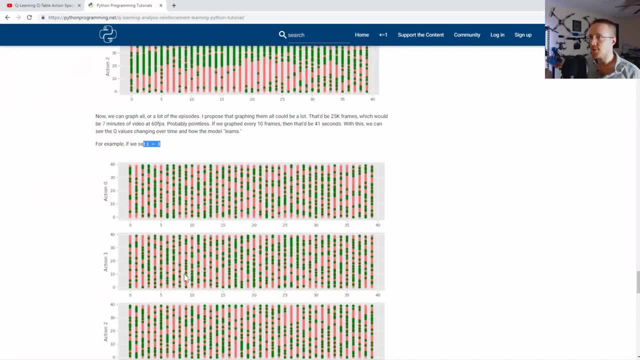 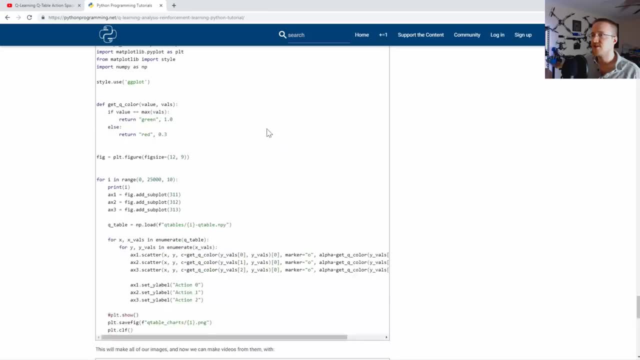 looking because it was randomly initialized. so you basically you go from here to here, which i kind of wanted to see happen. so i have all the cue tables. so then i use the following to basically iterate over all of the cue tables and save the chart. so i just made a cue table: charts. 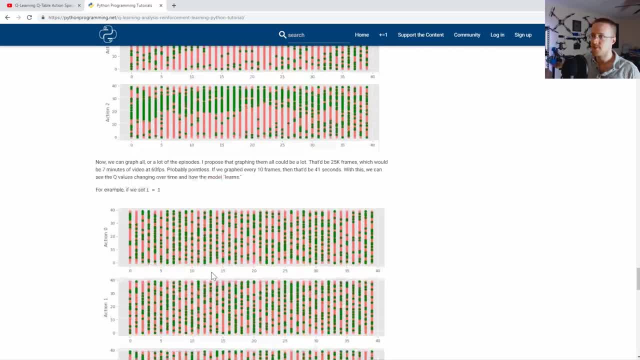 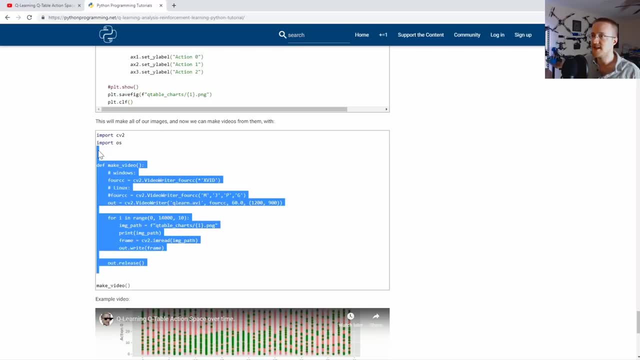 directory and saved every single cue table from basically from here to here in their graph form, and then the video code is here. it's the same code i use to make the deep dream stuff. if you haven't seen those, you'll probably just youtube deep dream syntax and you'll find it. 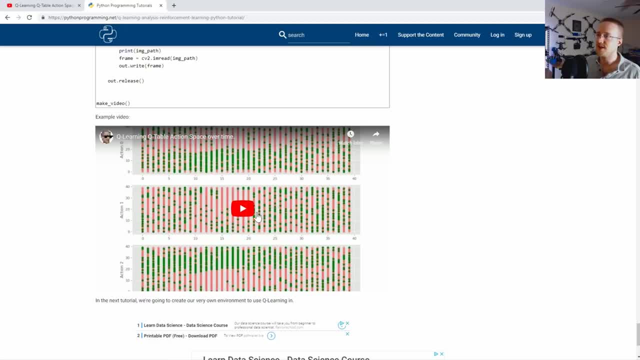 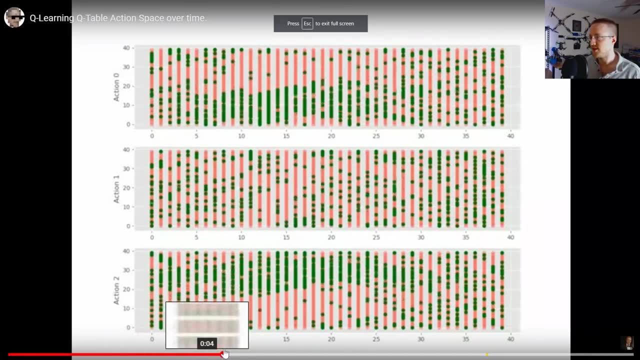 anyway, it's the same code from that and then we get a video of the cue table over time, which is pretty darn awesome. so this is it over time, and it goes kind of quick. i didn't really know, because the whole video is apparently this one's only 13 seconds, but i think i did 90 frames a second or 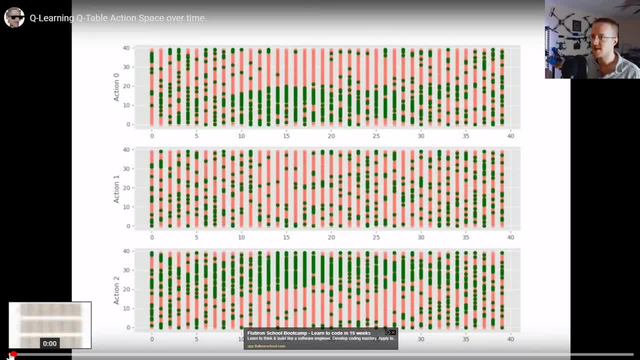 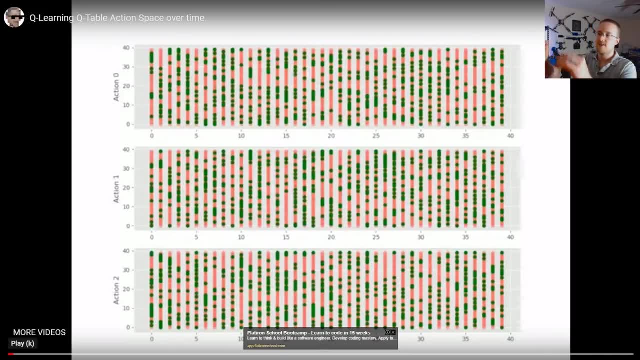 something like that, but it's not really something i want to stare at for the longest time. but it's kind of cool how you can kind of see how in the middle it- like it's obviously- starts random and then it starts like in the middle area of all the cue tables and then slowly expands out, which. 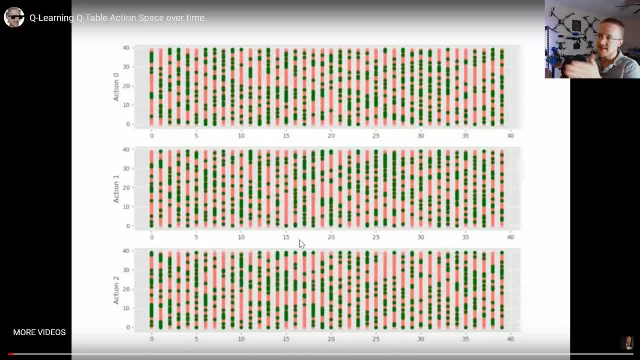 is kind of cool, um, because i guess that would be like: this is like the cart wasn't like a slightly off center position to start, and so i'm thinking it really is like left is, you know, left on these graphs, and then right is probably actually right on the graphs. i could be totally mistaken, but 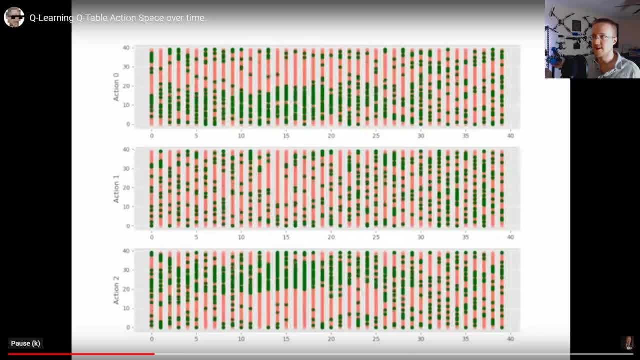 that's almost what it looks like, and then, as he continues to learn, uh, it continues to kind of fill out that entire space. but one thing you'll note is it never actually touches any of these like fully right positions, because the victory was at, i want to say, like 0.5, but the action space 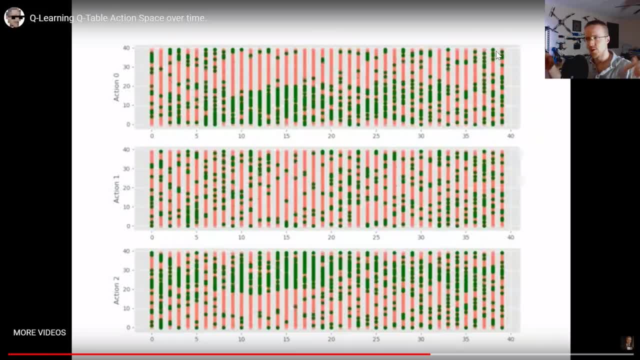 for that x-axis went to 0.6 or 0.7 or something like that, and i think that's why these never get touched, because the the car never goes to those positions. so it's kind of cool to to see it, because you can- you can actually see what's happening in the uh in the example on the graph, which is just 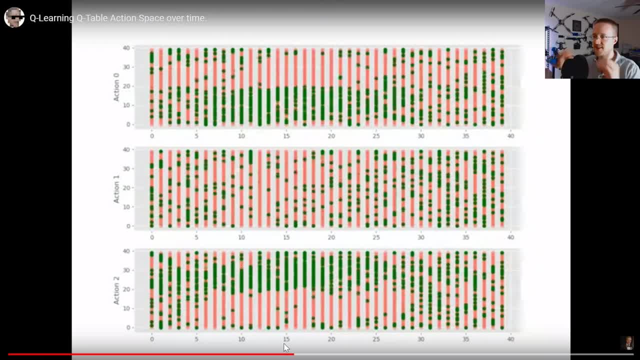 kind of cool, um, and also just the fact that it slowly grows out, and i think it's again, i think it's slowly growing out because it learns to push itself further and further by building momentum, and i just think it's super cool to see on in graph form. it's like, uh, staring at the matrix and 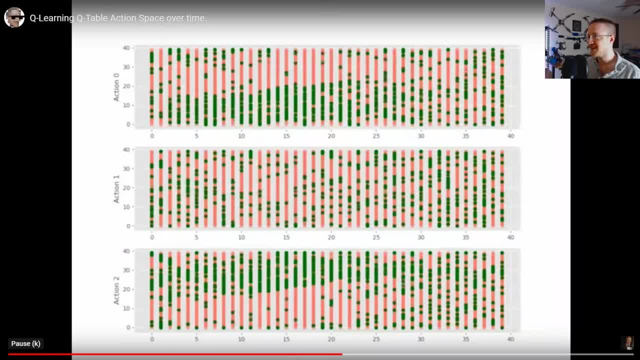 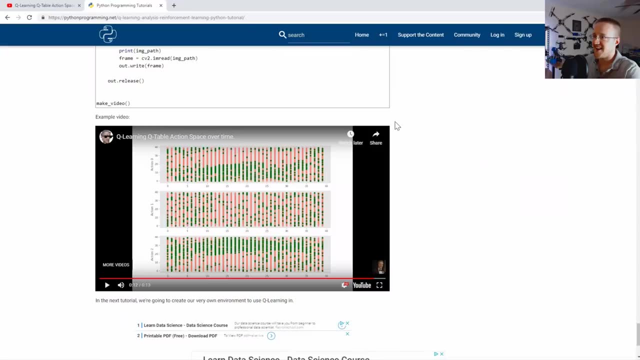 seeing, seeing the picture. so anyway, that's kind of cool, um, yeah, so, uh, feel free to make your own, or i think you can make your own, uh, and change the visualization, uh, if you want. this is just one way to do it. i still kind of want to make the 3d table thing, but i don't think i will. so anyway, uh, 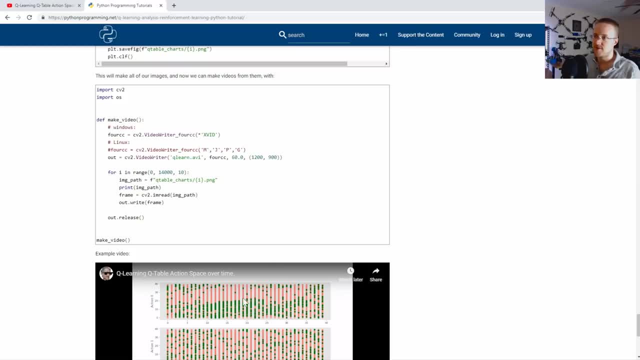 i think: yeah, that's everything for now. um, if you want, you can go to the text-based version of the tutorial and look at the video, or you can make your own video, change the colors, do all kinds of cool stuff. that's it for now. uh, in the next video, what we're going to do is build our own. 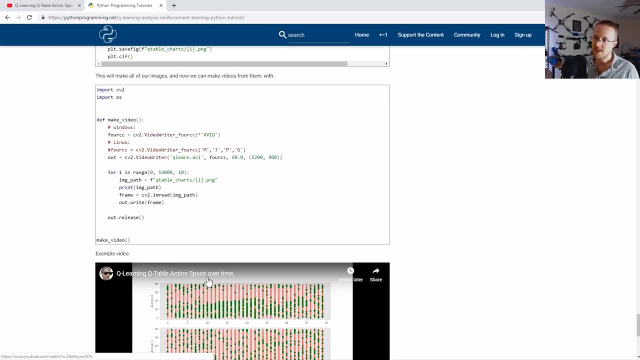 q learning environment. so q learning. the first thing i want to do is make my own environment. i i didn't really intend to do a tutorial on that, just because i didn't really see why, but everybody's asking about it and it's like so obvious like the first thing i wanted to do is build my own key learning. 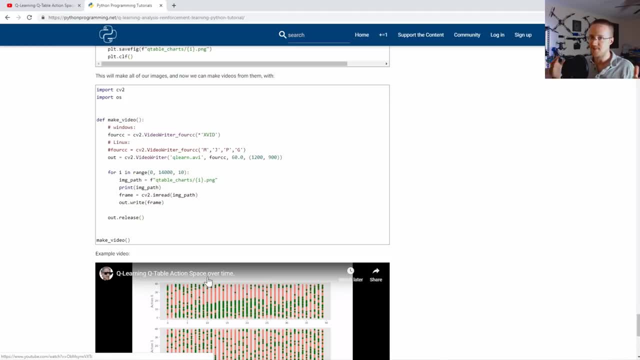 environment, so i guess i shouldn't be surprised that lots of people want to see us make our own, so, uh, so that's what i'm going to do in the next tutorial. and uh, the benefit there is that you can- if it's your environment, you can make certain tweaks and changes and, like, slowly, add complexity. 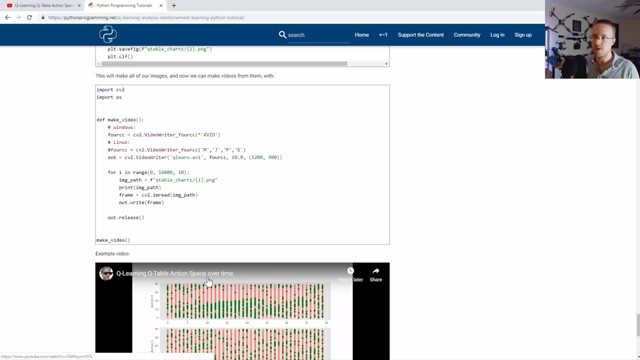 or remove or you know you, you have like full control over the environment, whereas, like with mountain car, i can't really make that environment too much more complicated. um, i could go with a different environment maybe, or something like that. but uh, yeah, you definitely have a lot of control if you can make your own environment. plus, you can start to 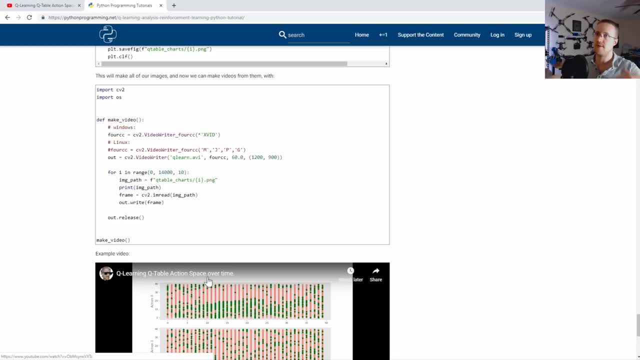 understand how you could take some like real world examples or maybe a game that you want to make on your own or whatever. so anyway, that's what we're gonna be doing in the next video- is actually making our own environment and then doing q learning on that environment. my hope is my. 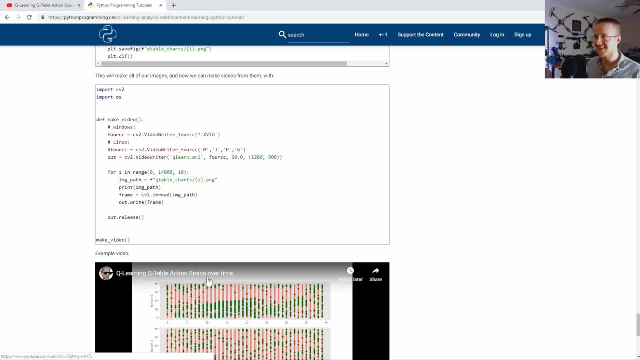 expectation is i can do it all in one video. so i hope you enjoyed the video and i'll see you in the next video. so it's gonna be the goal. so we'll see uh, questions, comments, concerns, whatever. feel free to leave them below if you want to hang out, ask questions and get- hopefully probably quicker.